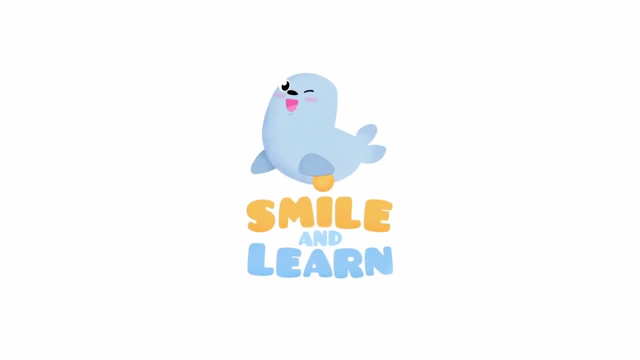 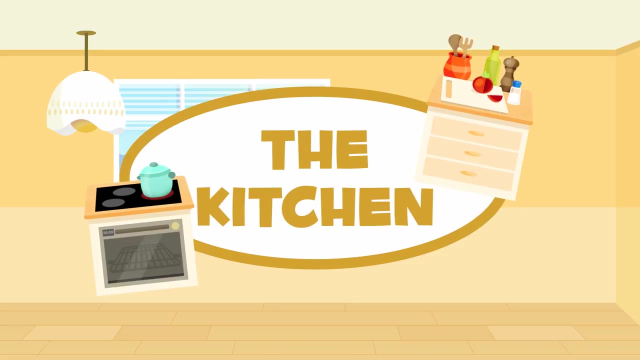 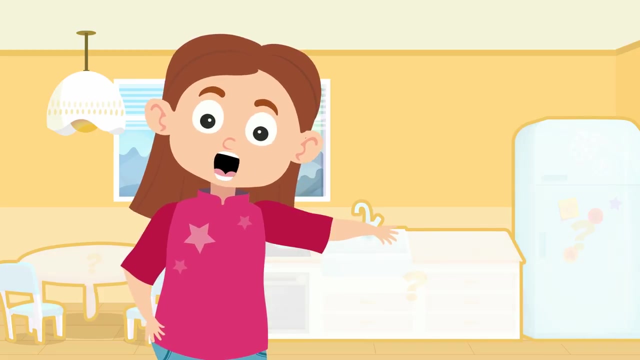 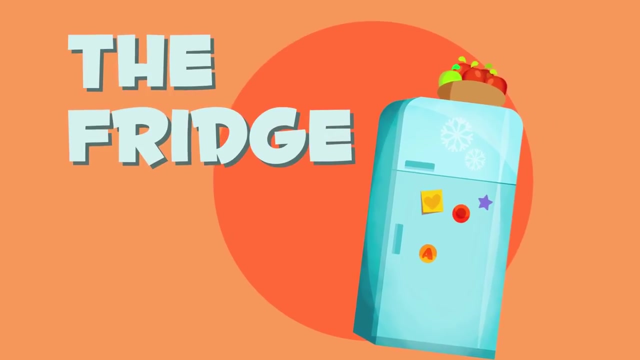 Today in vocabulary about the home, we will learn things about the kitchen. But what happened here? The kitchen is completely empty. We have to fix this. Let's add what's missing. Let's take a look at what we need: The fridge: We put fresh food in the fridge so it doesn't go bad. The sink: 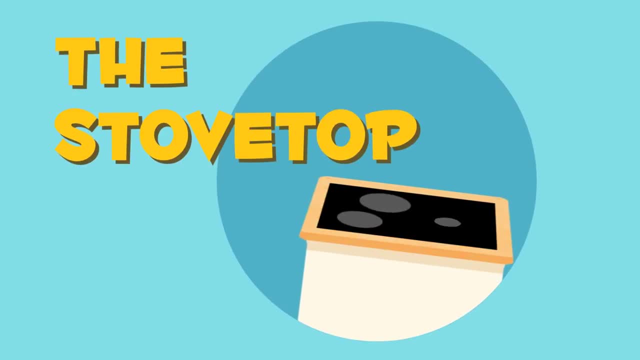 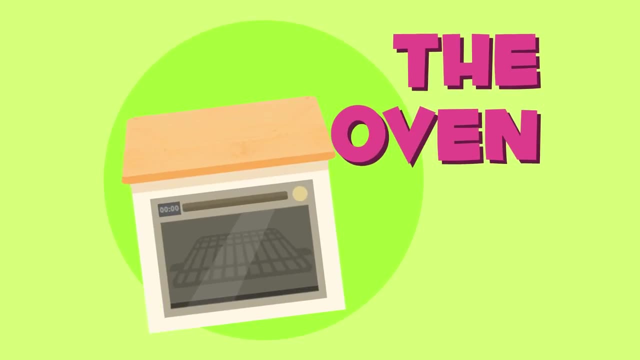 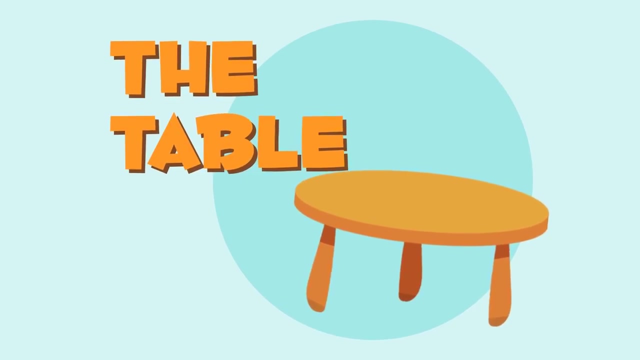 We wash dishes in the sink. The stovetop: We cook with pots and pans on the stove. Be careful, it's hot. The oven: We make pizza in the oven. I love it. The table: We eat at the table And we. 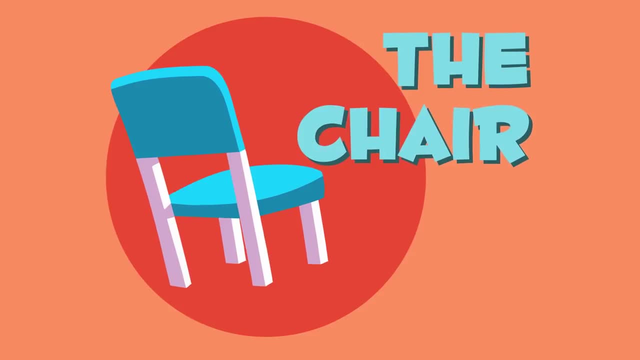 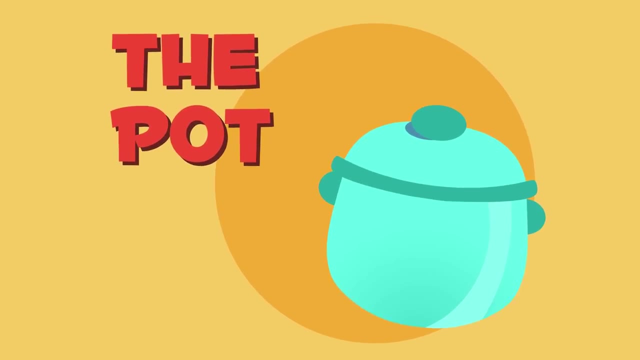 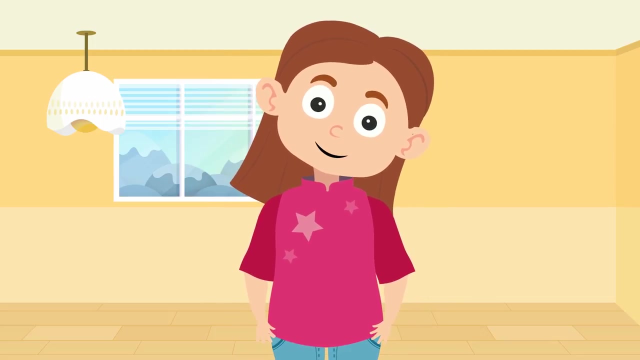 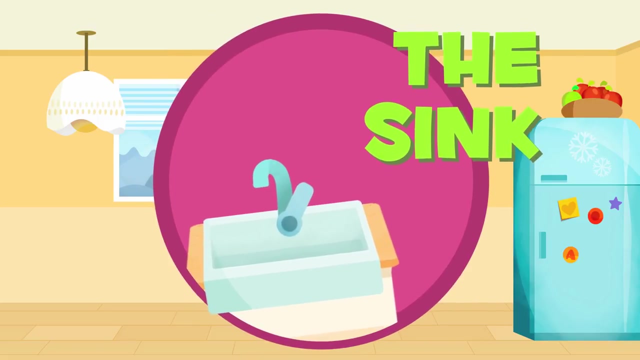 sit in the chair. Remember to sit properly when it's time to eat The pot. We cook our food in pots. Perfect. Now we need to put everything in its place. Will you help me? The fridge: We are going to put the fridge here. Great. The sink: Let's put the sink on the counter. The stove: The stove. 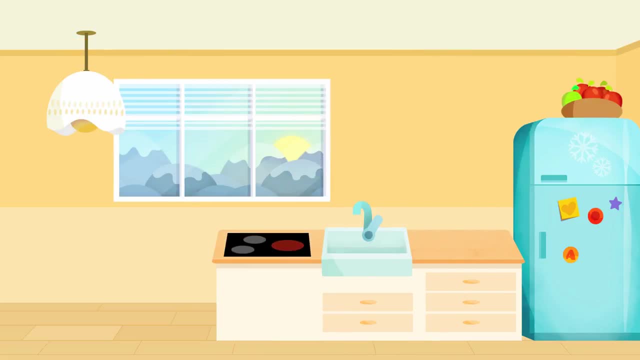 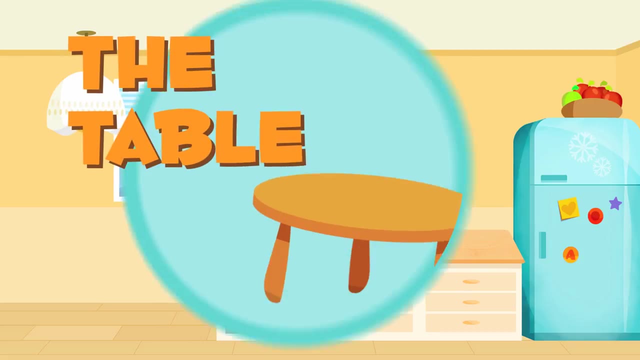 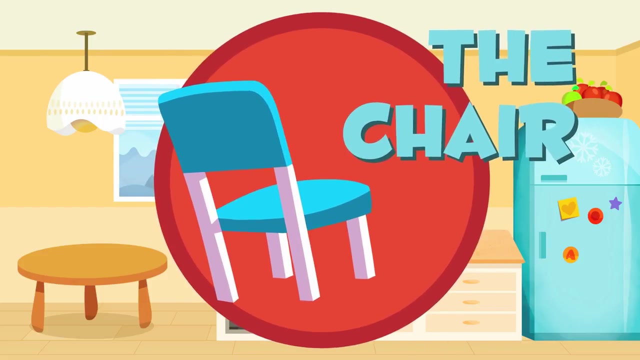 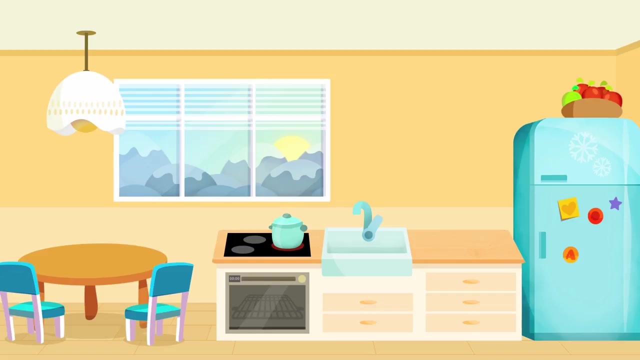 will go here to the left. Perfect, The oven: Should we put the oven under the stove? Fantastic. The table: Let's put the table right here in this area. The chair: Finally, let's put the chairs here beside the table. The pot: Let's put the pot on the stovetop. That way I can start getting dinner. 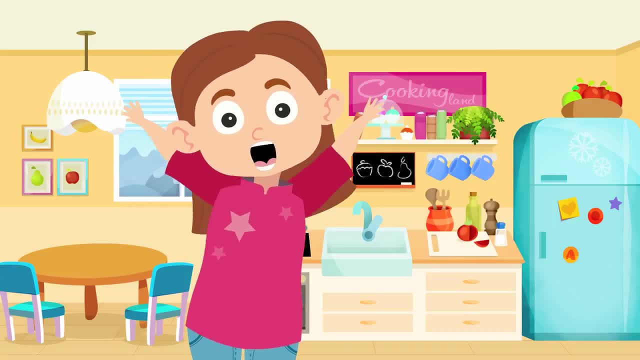 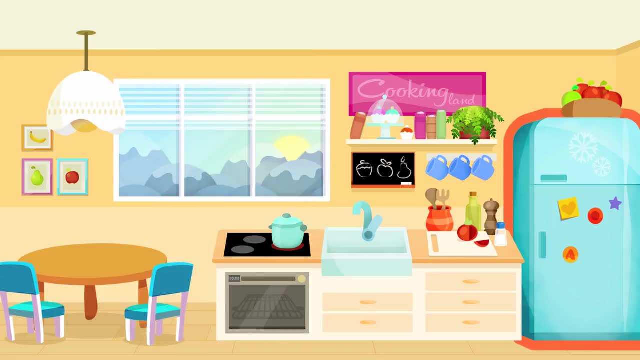 ready. That's it. We've got the kitchen. Let's review so we don't forget anything: The fridge, The sink, The stovetop, We eat dinner here And finally, let's put the table right. here We sit in. 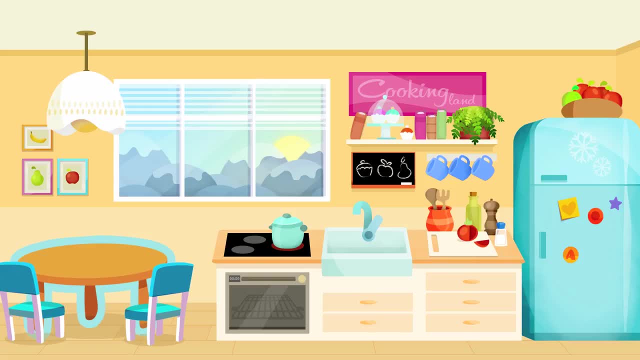 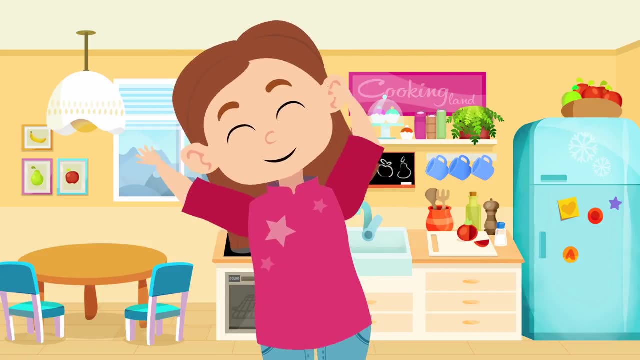 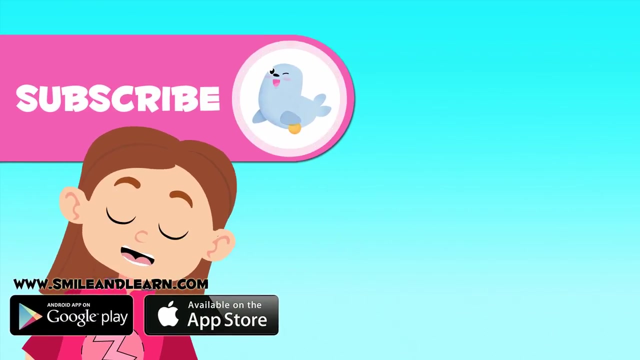 The oven, The table, The chair, The pot. Yay, Great Thanks for watching.